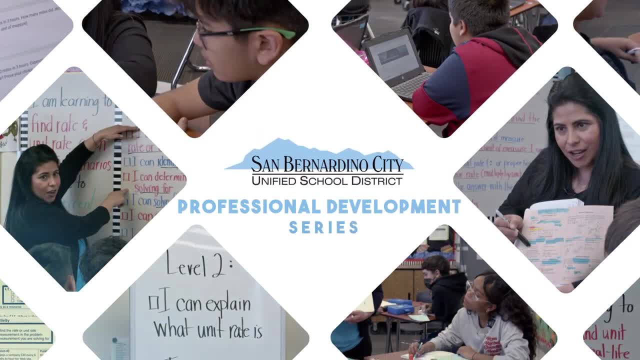 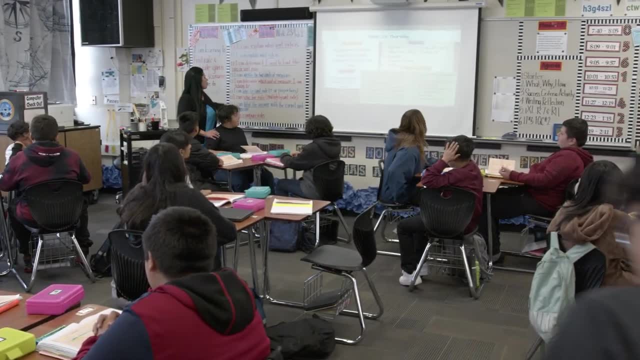 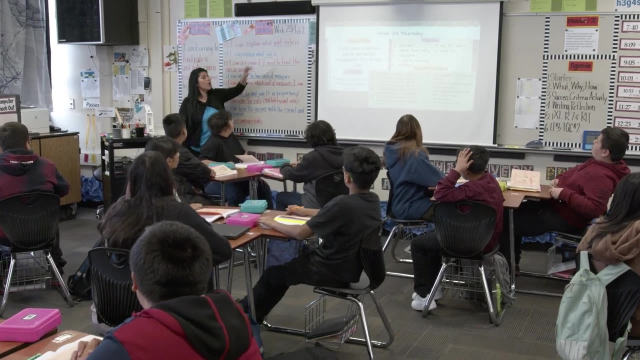 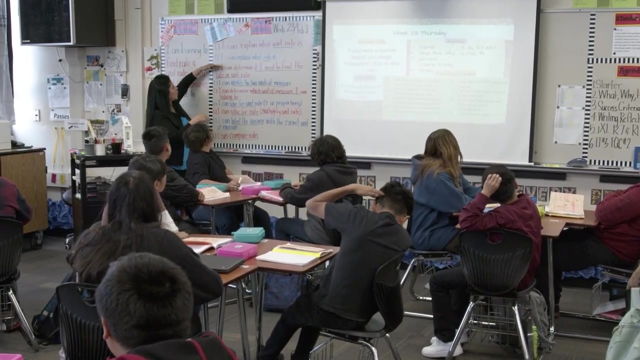 Our first activity is going to be based on these two success criteria. So what words are you going to be talking about? Okay, Our second level, three. okay, that activity is going to be based on three of these success criteria, right here. Okay, And what two terms are you going to talk about? 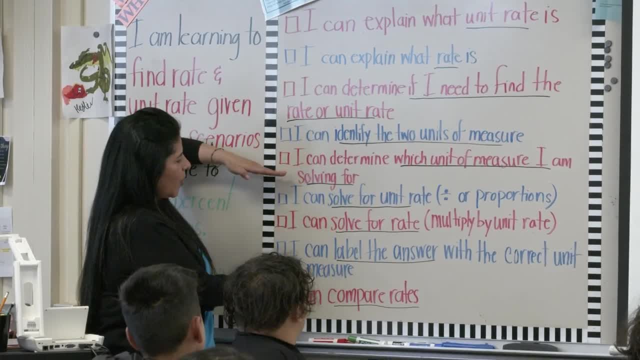 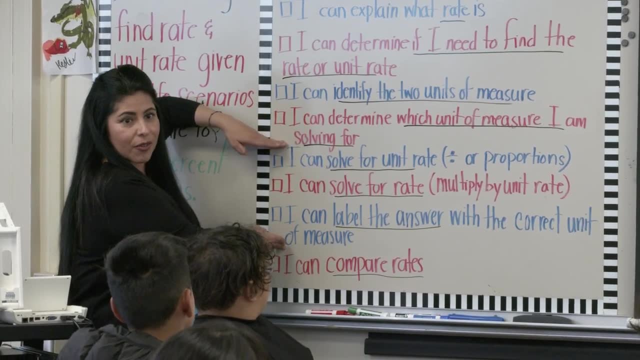 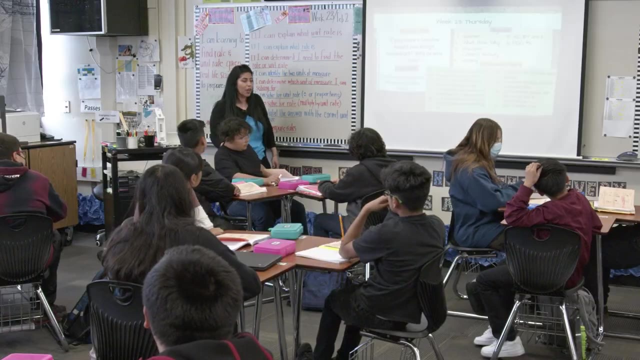 Rate and unit rate, Okay. And then we have another activity, a level four activity, based on these success criteria. What two words are we going to be talking about? Rate and unit rate? And then our last activity is a level five and we're going to be comparing rates. Okay. 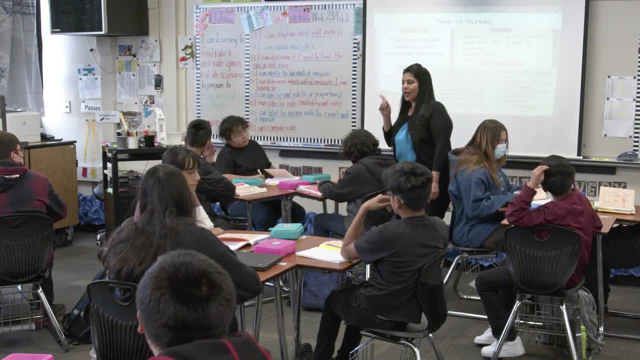 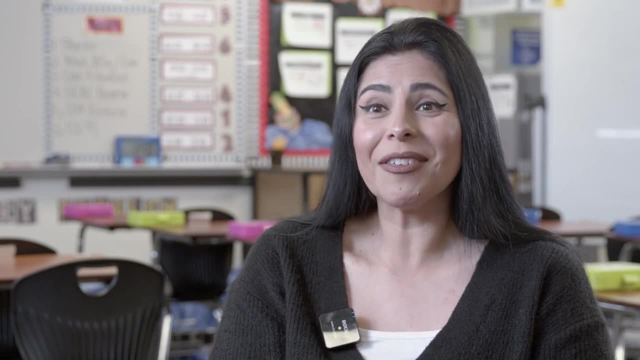 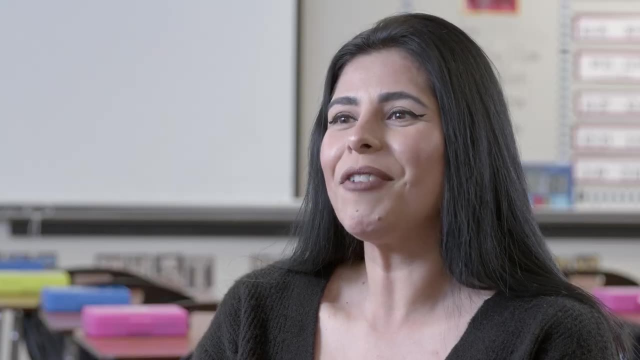 You are more than welcome to use your notes. Writing success criteria for student success is very important because not only does it give them a clear map as to where they need to go and how to get there, but it also puts the learning onto their plate, So they become the. 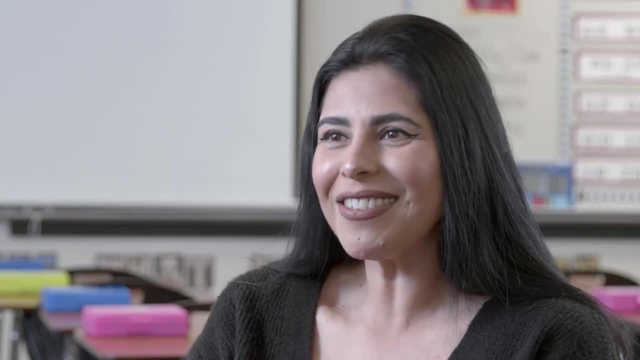 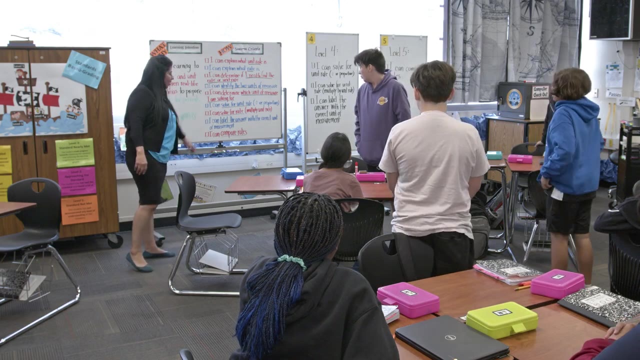 facilitators of their own learning. rather than me teaching and them listening, They're learning through functioning with the success criteria We talked about. we can solve for rate. What's the next thing that we're going to be able to do? I can label the answer with correct unit of. 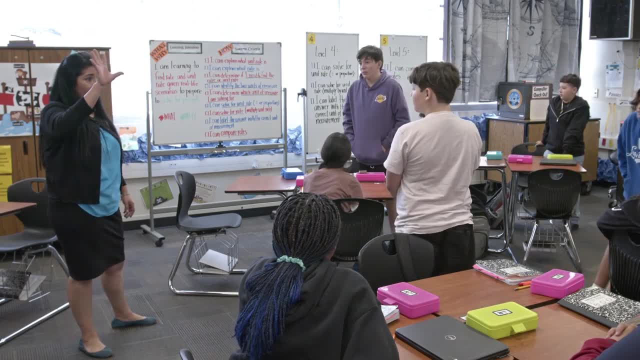 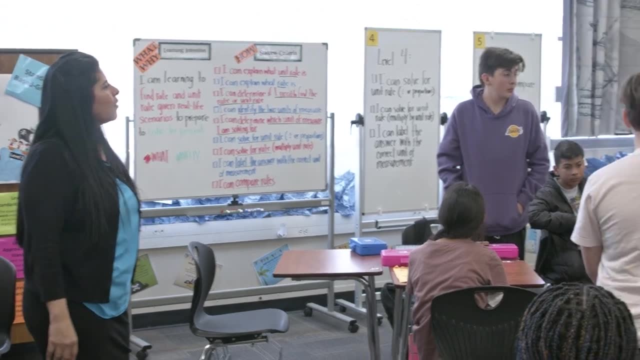 measure Excellent, So you should be able to label your answer. Don't just put five, but five miles or five dollars or whatever. it is just like Jojo and Nico talked about. What's the last thing we should be able to do On a daily basis? the students will look at three. 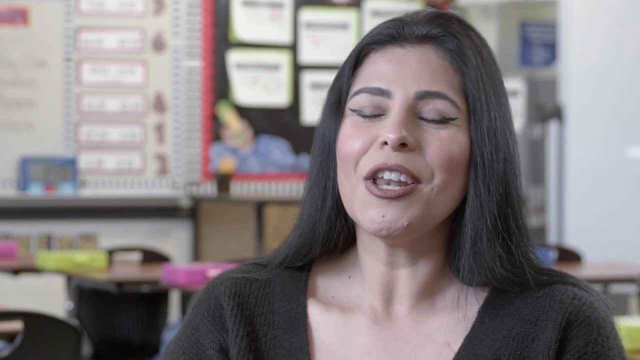 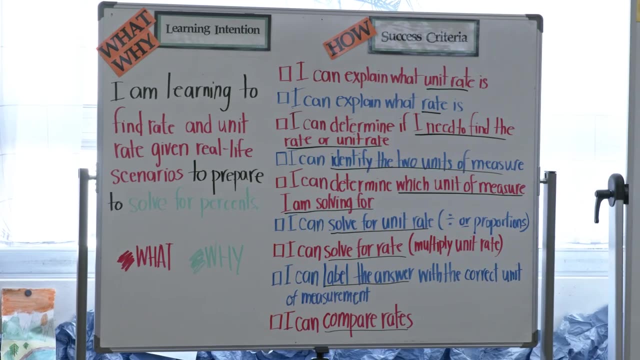 pieces of information before we get started into activities. Number one, looking at the learning progression. Where are we at in the unit? Number two, looking at reading and discussing the learning intention. So what are we learning for the day and why are we learning it? And then number three: 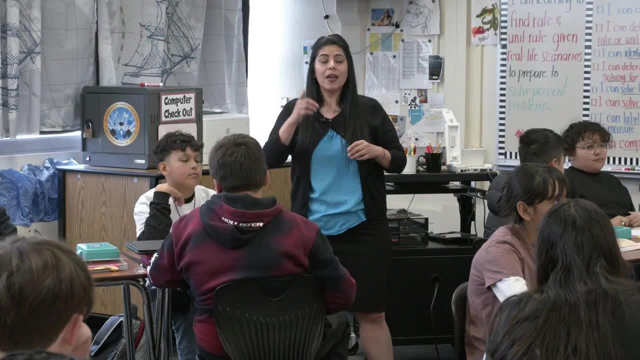 how do we know if we've learned? which is the success criteria? Right, Let me show you. My level two is back here. Okay, This is where everybody's going to be able to learn and they're going to be learning. Okay, This is where everybody's going to be learning. Okay, This is where everybody's going. 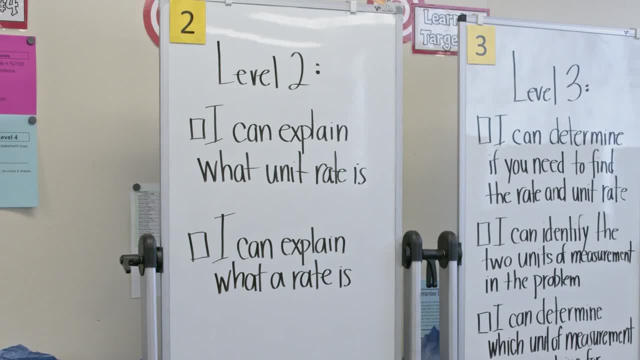 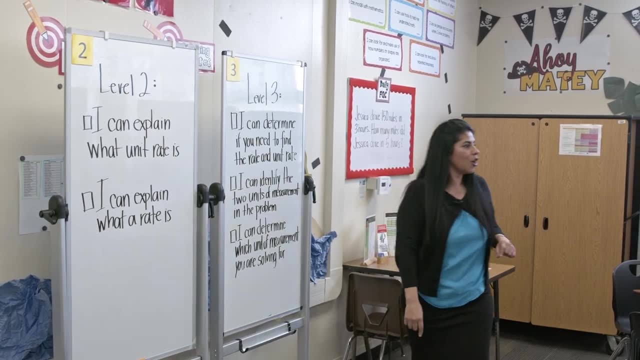 to start with a level two, and it's going to be based on these two success criteria, And then you're going to move to a level three based on these three success criteria, and the papers are right down there. Where's level four? at Right here. Okay, Level four is based on these success. 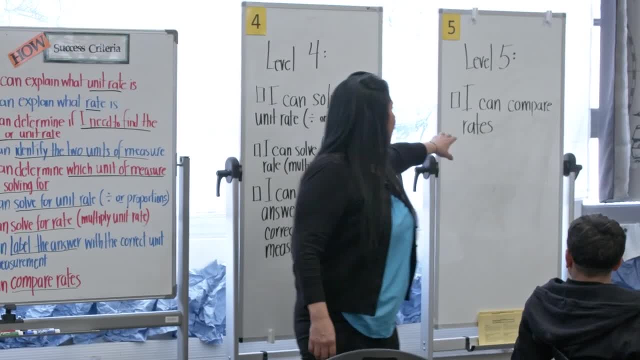 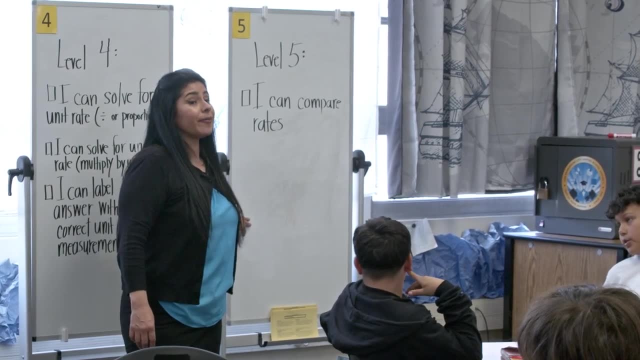 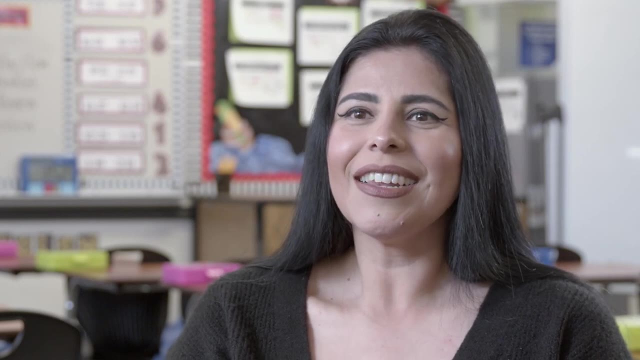 criteria and the papers are on the floor. And then level five is based on the last success criteria and the papers are right there. Okay, How many papers do you grab One per? So the activity for the day was based on the success criteria for our particular learning progression we're working on- And I broke the four activities. 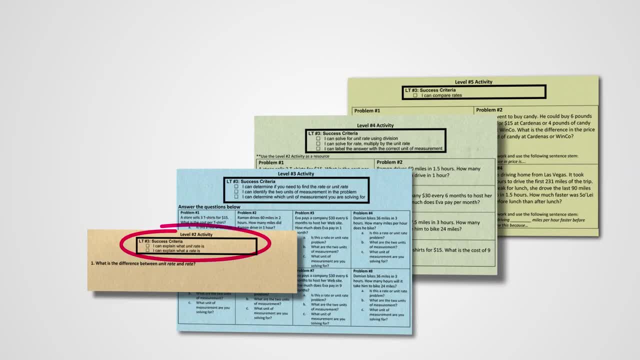 up into levels. So the first level was based on the first two success criteria. The second level was based on success criteria three through five. The third level was based on success criteria six through eight, And then the last level was based on success criteria number nine, If you were to. 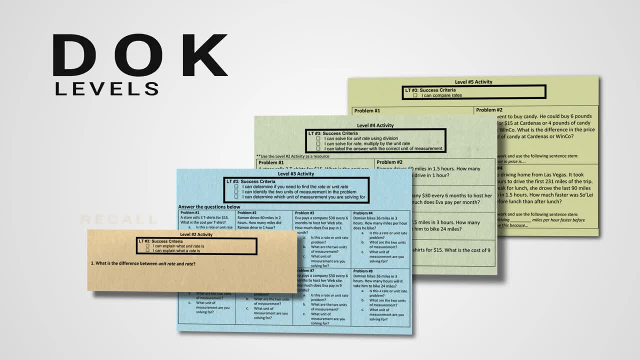 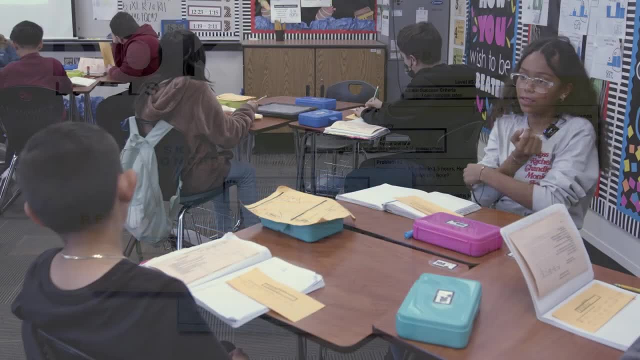 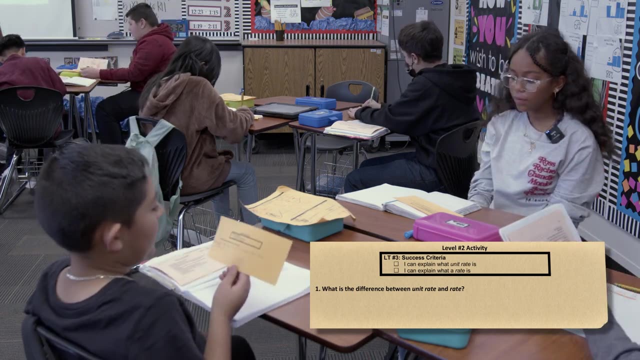 look at our success criteria. it begins with a DOK one and then begins to build up. So something very simple to something that requires application. So what did you write Like? well, the difference is unit has per one inch and rate does. 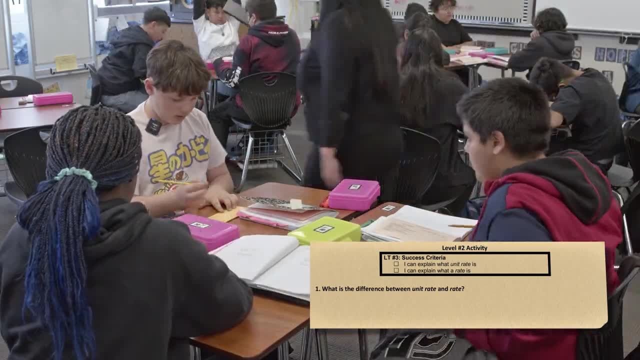 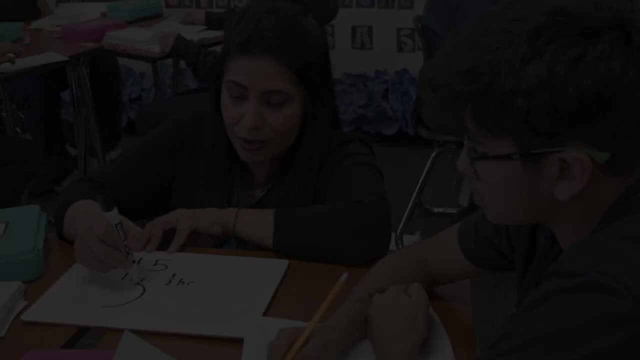 Yeah, Okay. So unit rate and rate. Unit rate is it's like it's exactly like rate, but it's using one. So let me say so, this is one hour. Yeah, Okay, How many minutes is that? 60., 60. And this is. 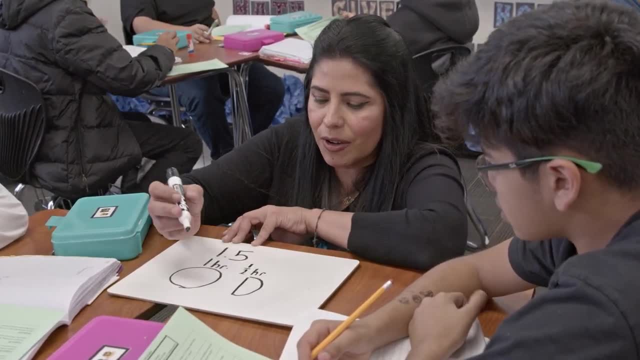 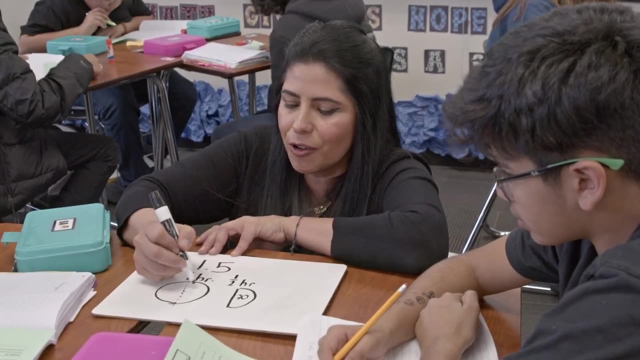 half an hour. Yeah, How many minutes is that? 30., 30. Okay, So let me ask you this: What if I took this clock and I broke it in half? 30 and 30.. 30 and 30. Which equals what? So questioning is really. 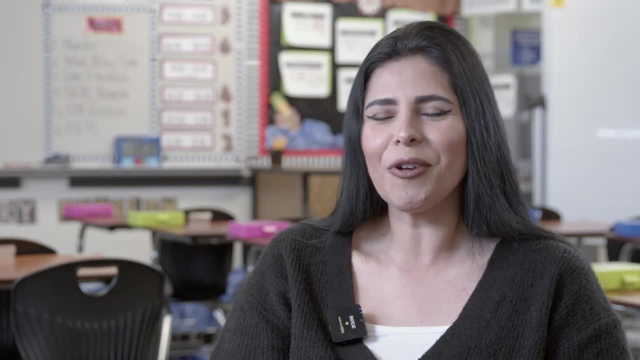 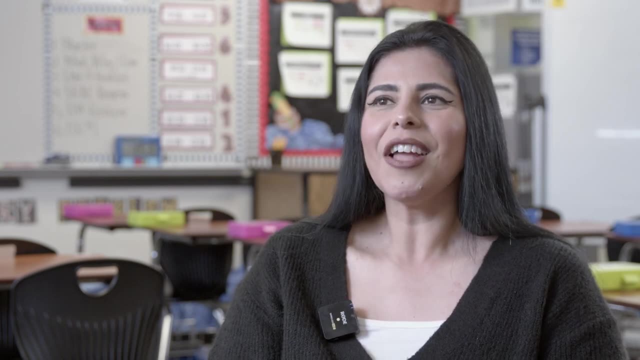 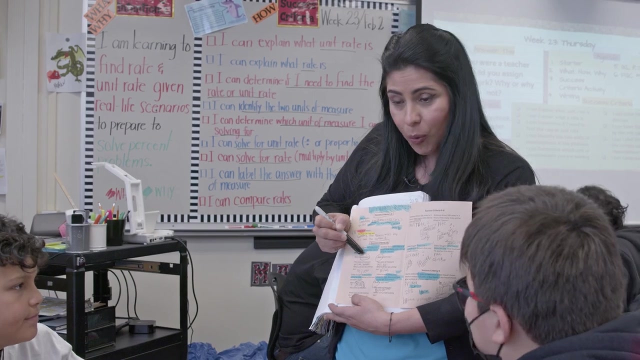 important, especially on day two of a particular learning progression, And what you're seeing here in this particular lesson is me facilitating, not me giving answers, not me saying right or wrong, but asking questions so that students can think through their their own thinking and their own work and begin to develop questions that they can ask one another. 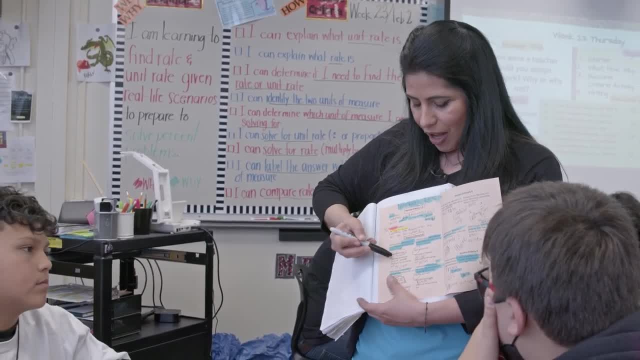 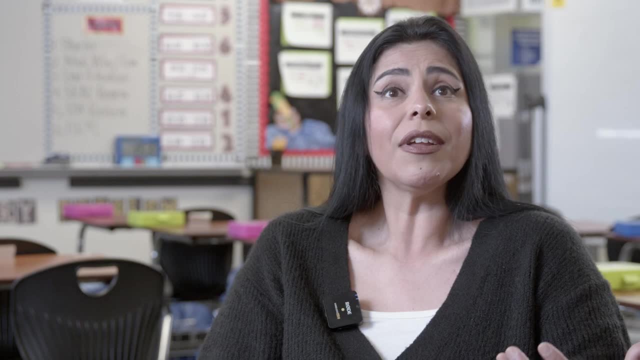 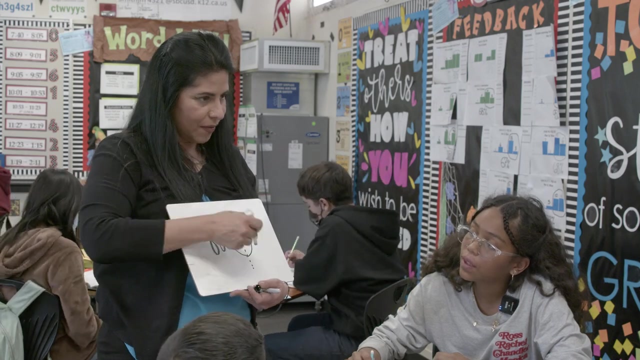 So the goal of asking questions is to facilitate learning, so that they can collaborate together and determine the answer or to a problem, or even determine whether they're on the right path to finding that answer. Okay, So what would half that time be? Okay? So here's 30 minutes here.